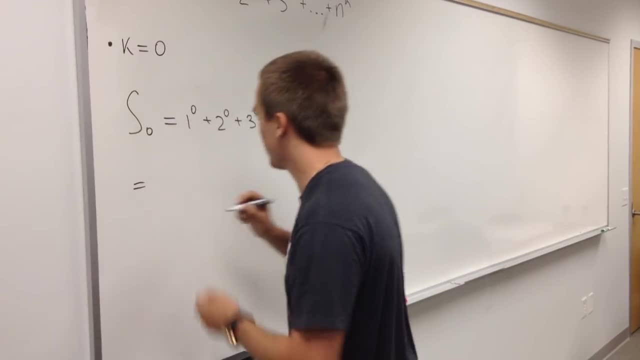 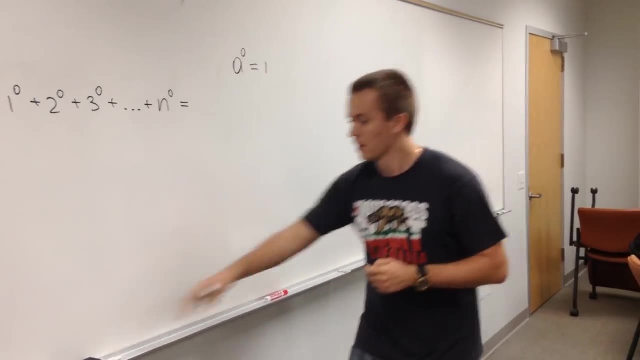 And you can see this is really simple and trivial. Why? Because if you have number a and number a to the power of zero, it's just going to be equal to one. So in this case, each of these terms is going to be equal to one. 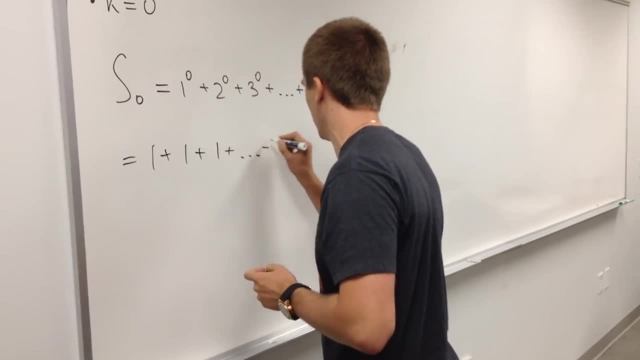 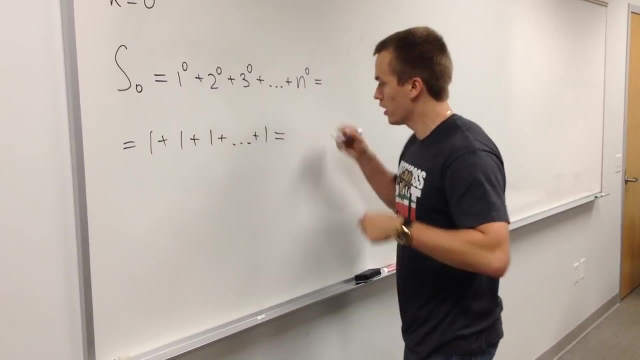 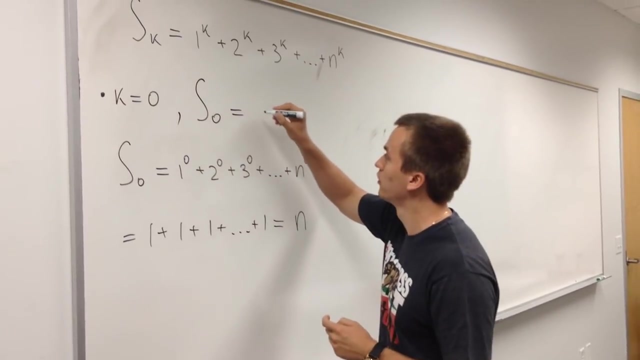 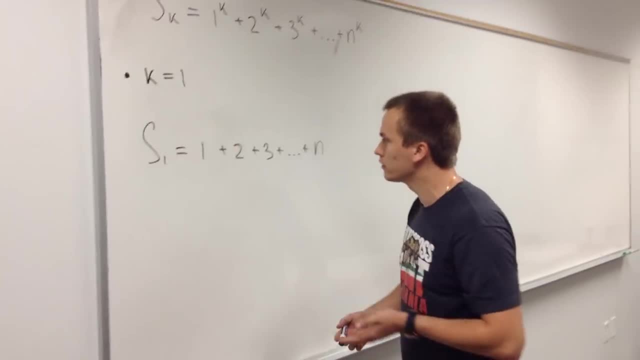 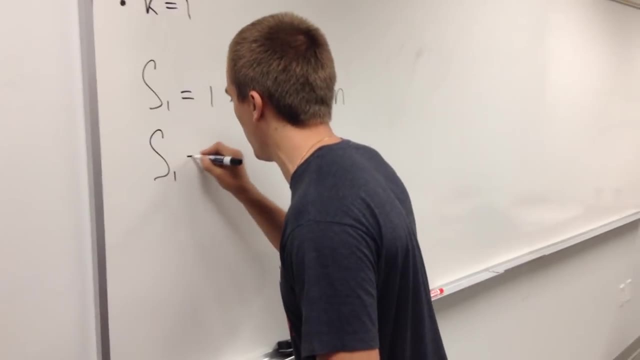 So in a case when we have k equal to one, I will prove this formula by using one really interesting trick. So what I'm going to do? I will write the same like s equal, But here I will change the order of my terms. 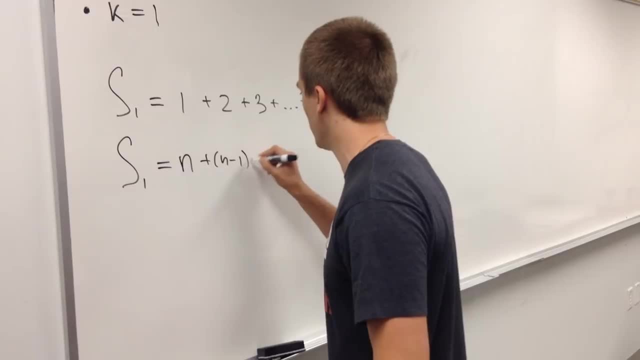 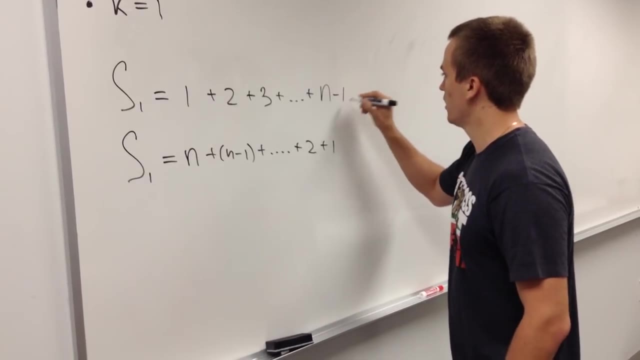 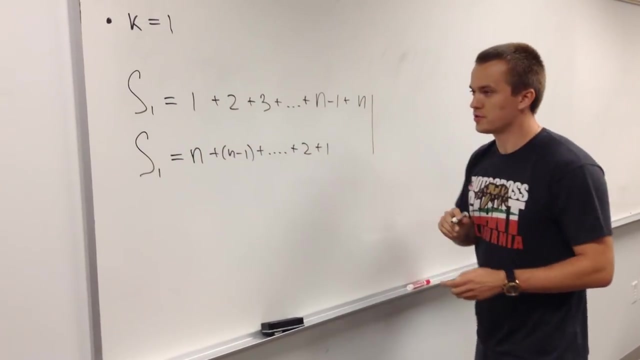 So I will write down this: n plus n minus n, And I will write n minus one plus ta ta ta plus two plus one. So in this case I will just write n minus one plus n And what I'm going to do when I have these two sums, I'm going to add them up. 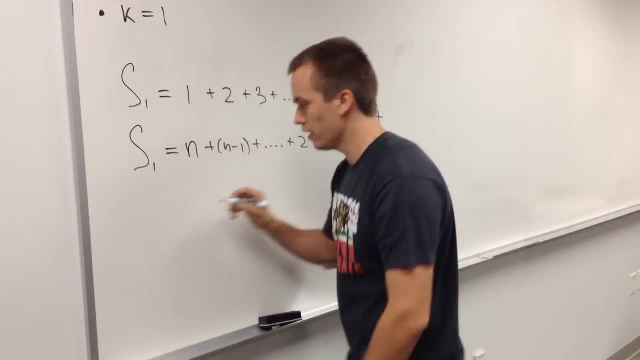 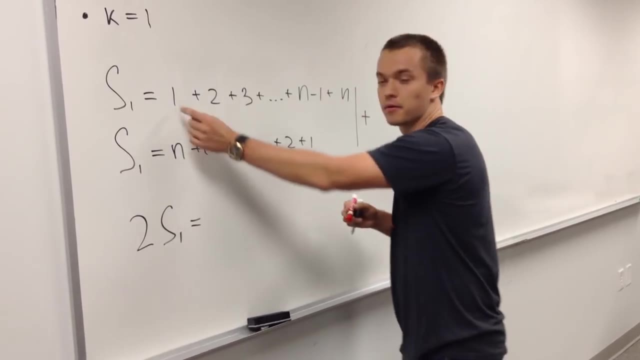 So in this case, you can see: if I will add s one plus s one, I will get two s one. But what I will get for each of these terms you can see. if I will add n plus one, I will get, as a result, n plus one. 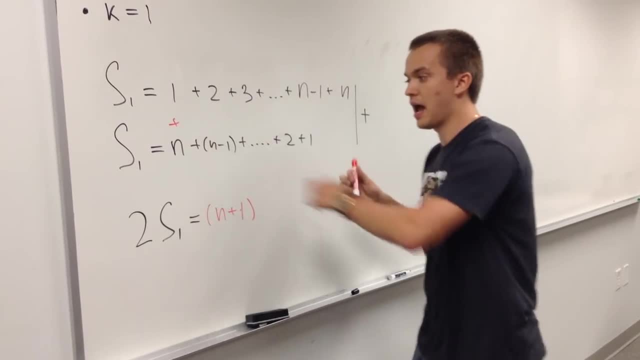 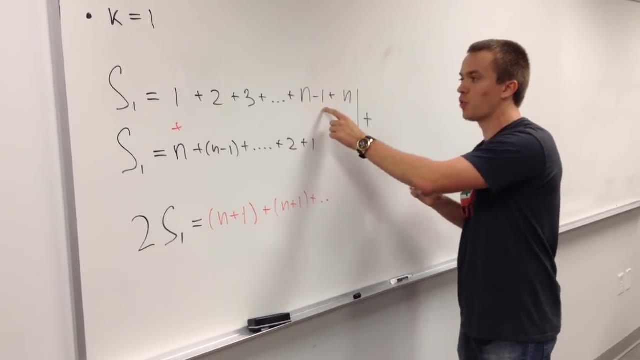 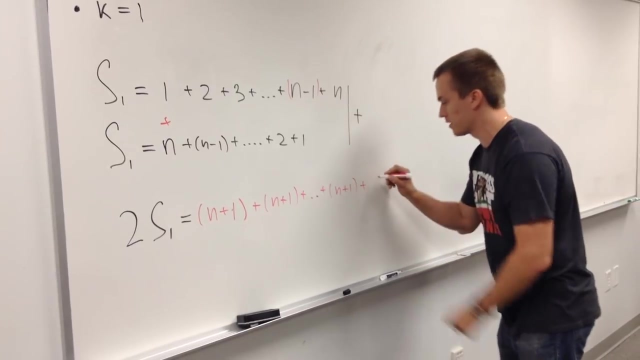 Yeah, If I will add two plus n minus one, I will get n plus one, And so on. If I will get n minus one plus two, I will get n plus one, And the last term is going to be also n plus one. 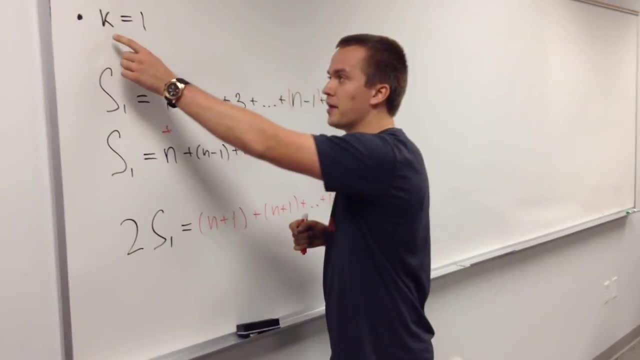 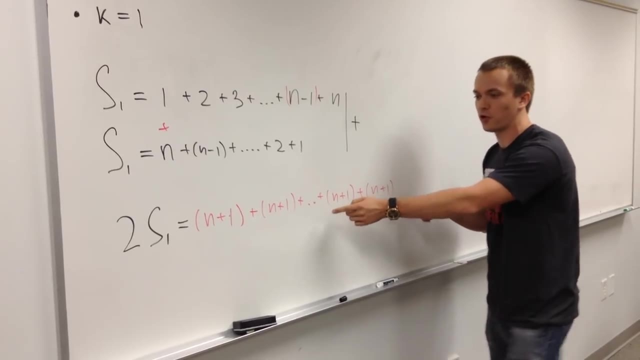 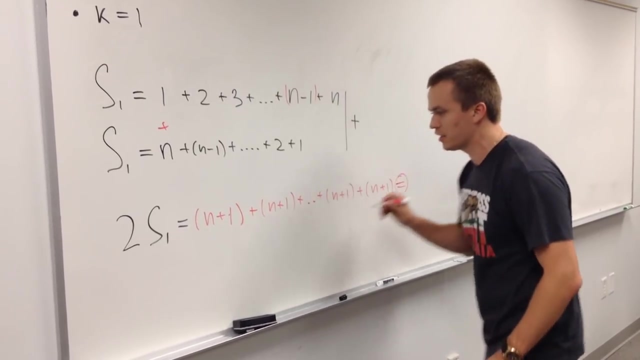 And right now you can see, by finding the sum for k equal to one. I made the same approach when I was looking for s zero. Why? Because right now I have n equal terms, So all these terms is going to be equal to n times n plus one. 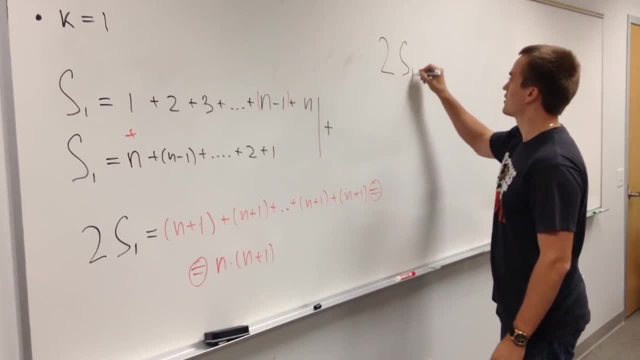 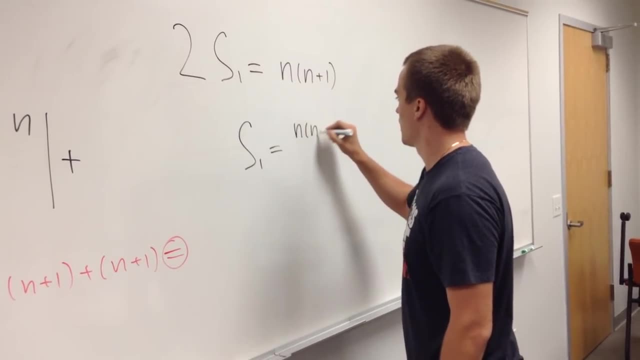 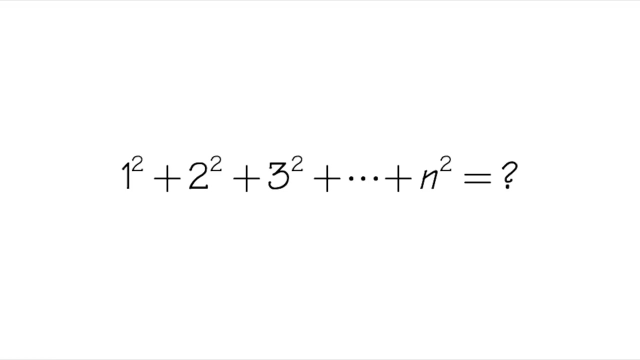 So what I get? I get that two s one equal n n plus one. I can see that my s one is equal n? n plus one over two. So we got our result for k when k is equal to two. And let me prove this formula: when k is equal to two: 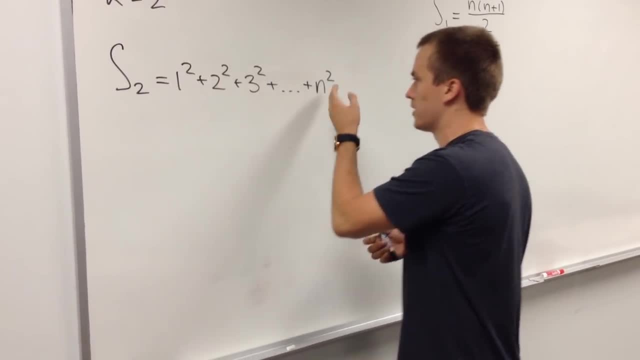 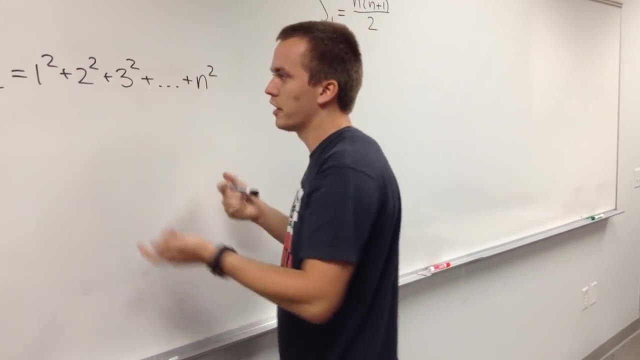 So in this case you can see you have one square plus two square, plus three square, dot, dot, dot and plus n square. And what can I do? If I'm going to change the order, it's not going to help me. 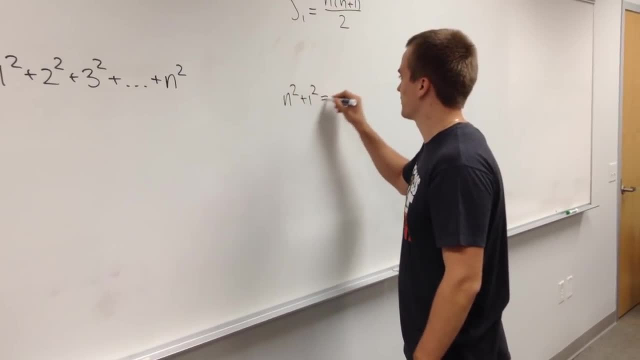 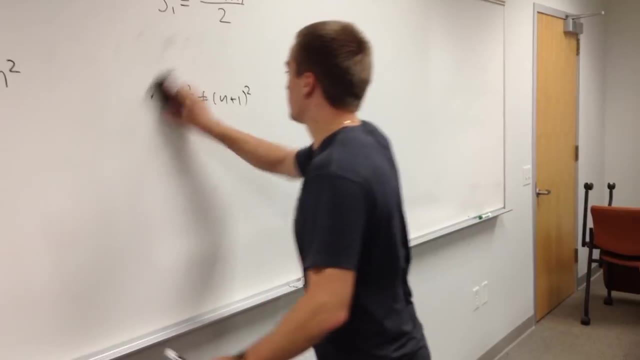 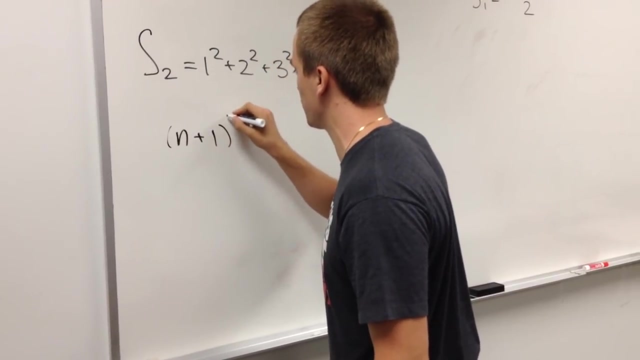 Why? Because n square plus one square doesn't equal to n plus one square. So I cannot use this method. But what I'm going to use? I'm going to use another trick. So what is this? what is this trick? Let's consider this expression: n plus one cube minus n cube. 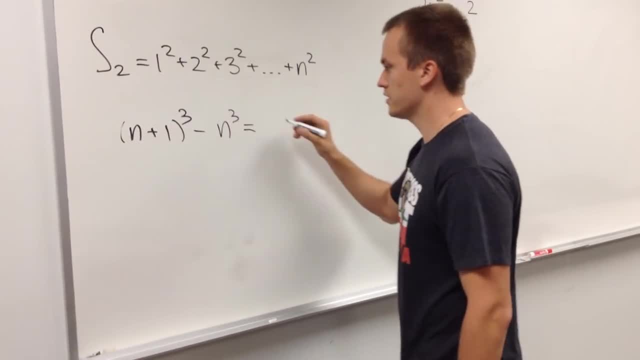 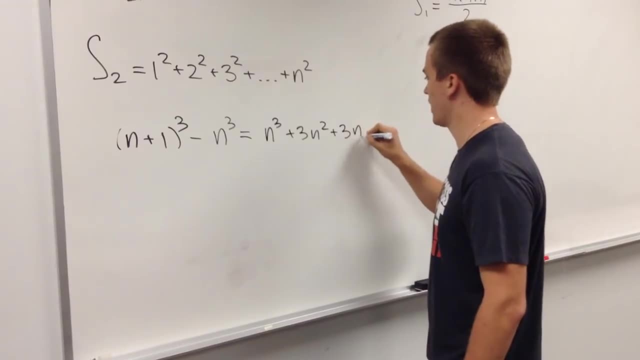 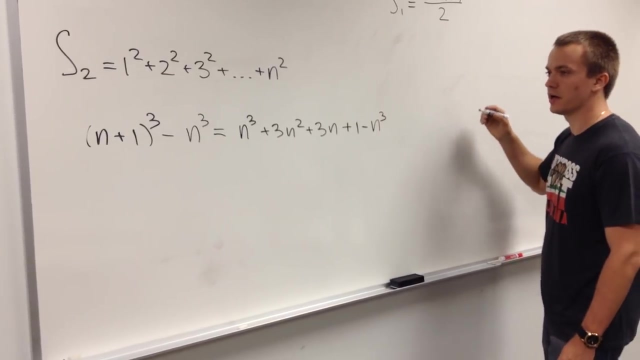 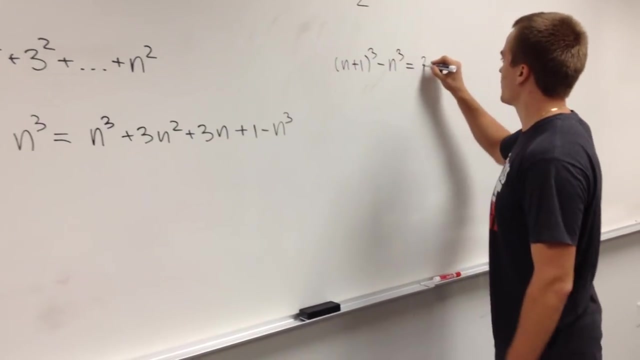 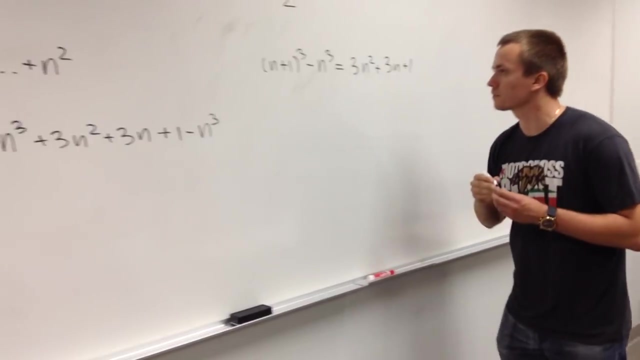 Let's find what is this equal to? And this is equal to n cube plus three n square plus three times n plus one minus n cube. So you can write this down as n plus one cube minus n cube, equal to three n square plus three n plus one. 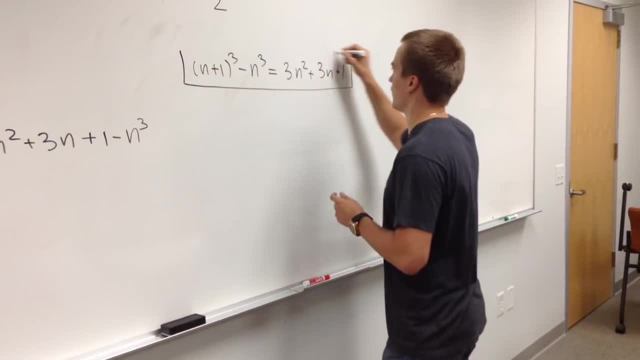 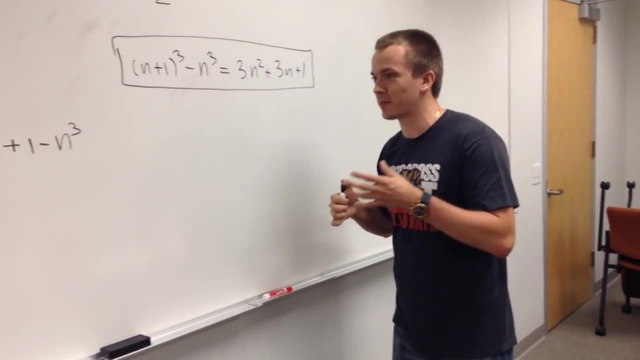 So you see, we got this formula And you maybe ask yourself how are we going to use this formula? And again, we are going to use some kind of ordering and some kind of manipulation of these objects. So what I'm going to do, 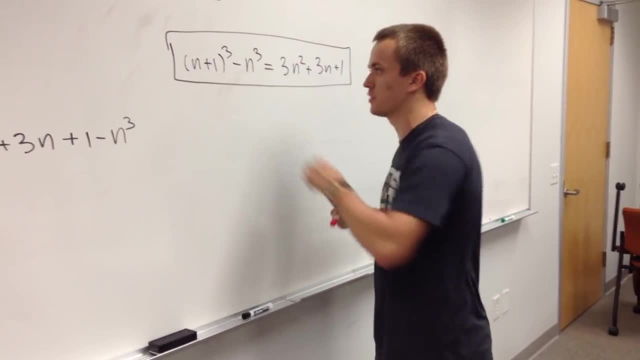 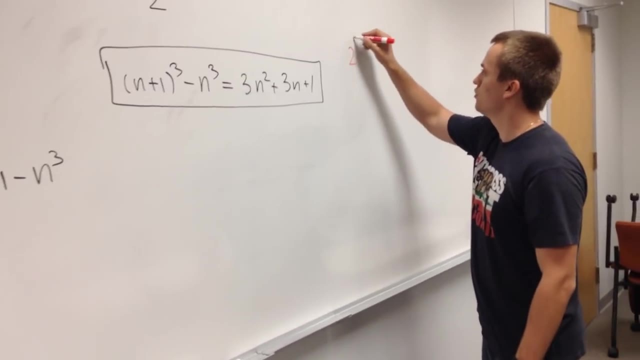 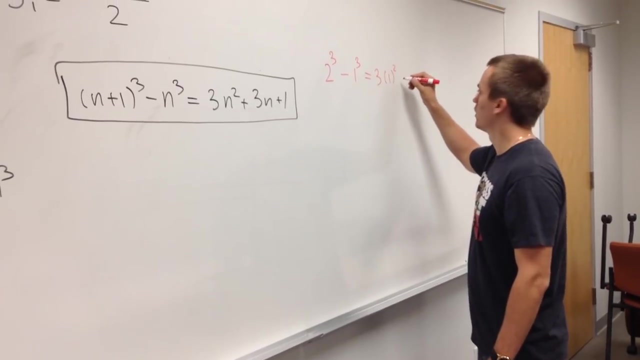 I will take some cases for this: n. So let's write this down: when n is equal to one. So when n is equal to one, what will we get? We will get two cube minus one cube equal three, one square plus three times one plus one. 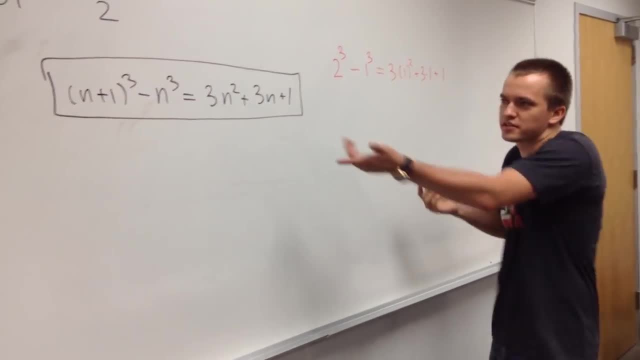 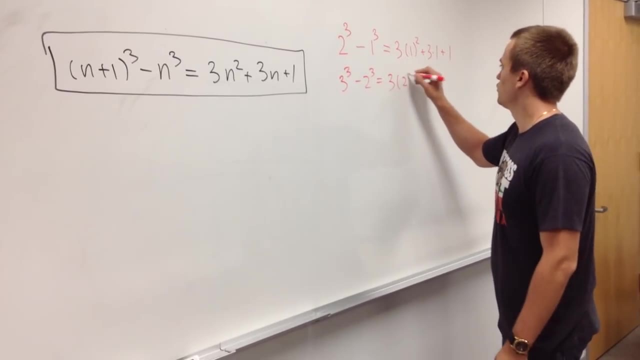 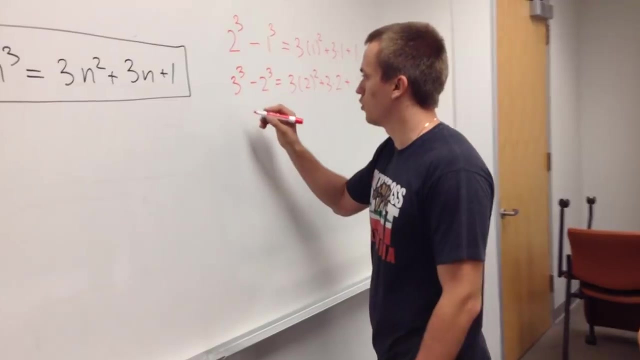 Okay, good enough. So let's write this down for n equal to two. So what will we get? We will get three cube minus two cube equal three, two square plus three times two plus one. And let's do one more for n equal to three. 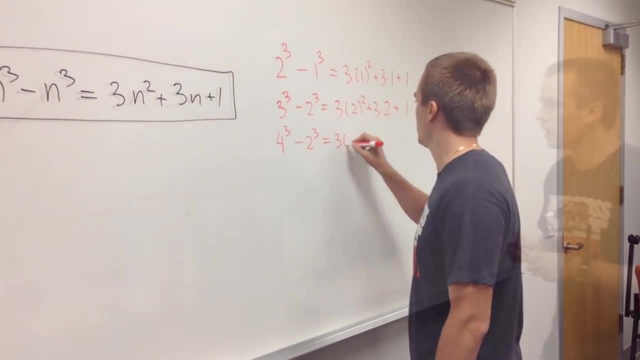 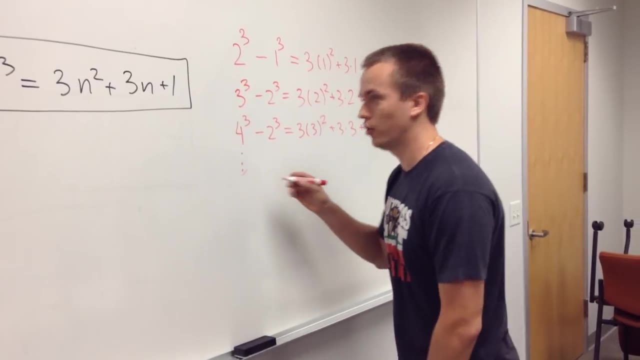 I will get four minus two cube equal three. And let me do like this in a case when n is equal, for example, to m minus one. So what will I get? I will get m cube minus m minus one cube equal three. 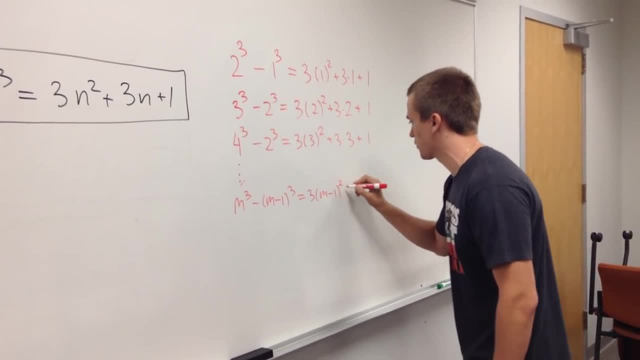 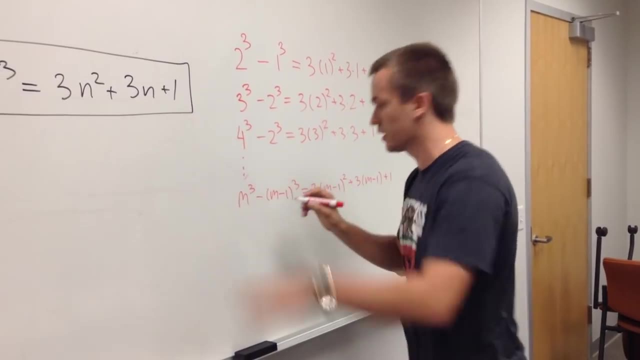 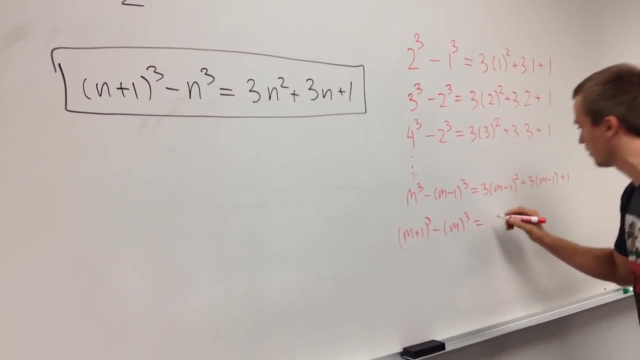 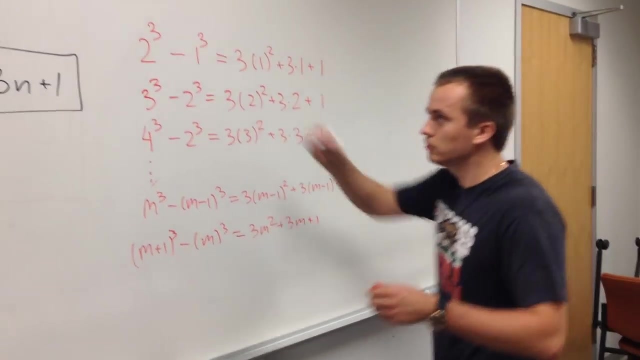 m minus one square plus three m minus one plus one, And our last term is going to be n equal to m. I will have m plus one cube minus m cube equal three m square plus three m plus one. Okay, I got this table. really nice table. 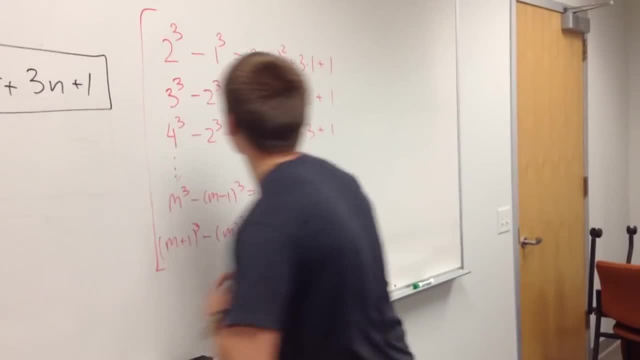 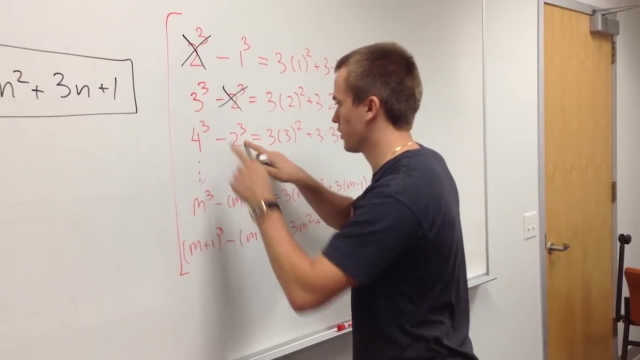 And right now I'm going to do magic. So what is magic about? It's about okay. so I have two cube and negative two cube. I will cancel them out. I have- oh sorry, it's actually three, Yes, two minus three cube. 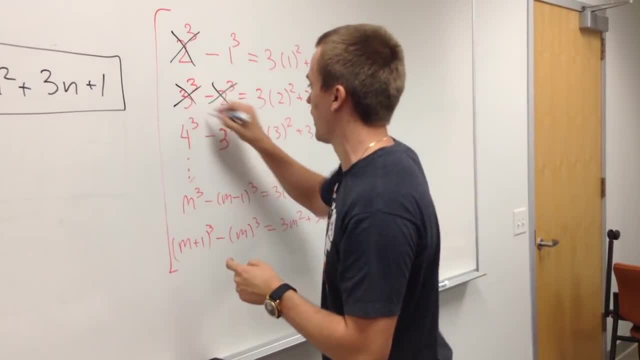 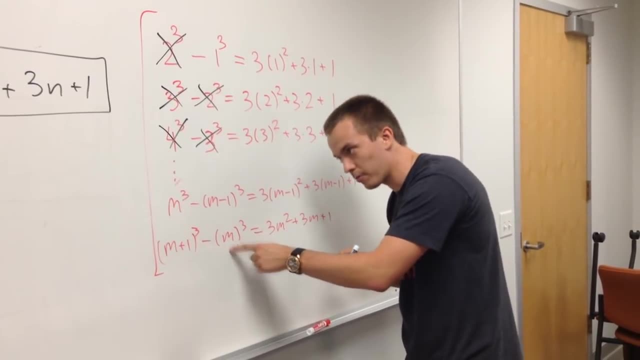 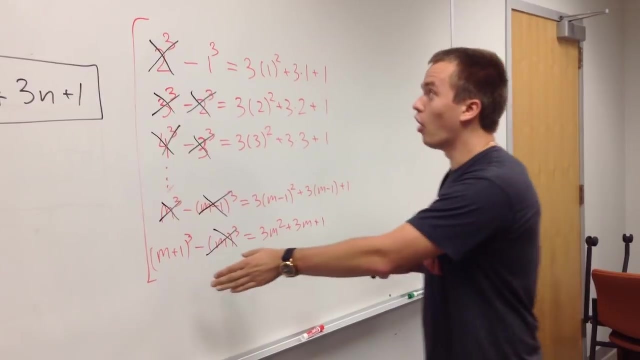 I have three cube negative. three cube: I get cancel out. Four cube negative. four cube: I get cancel out. m m cube minus m cube Get cancel out. And negative and this term also get cancel out. So on the left side, 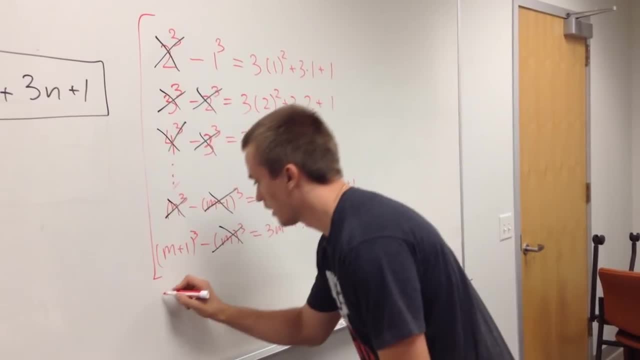 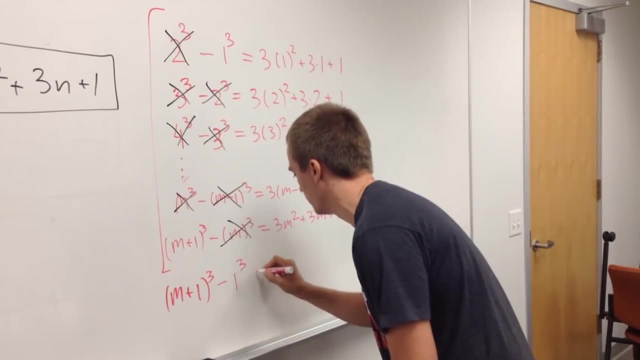 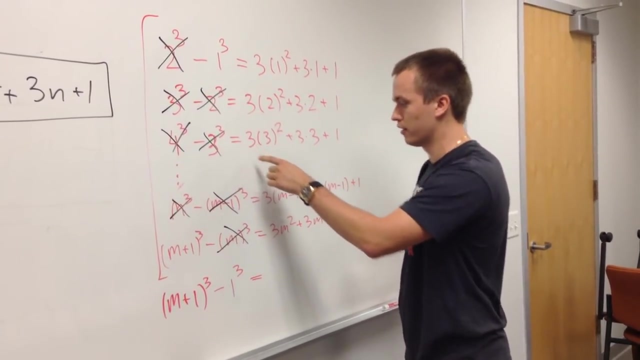 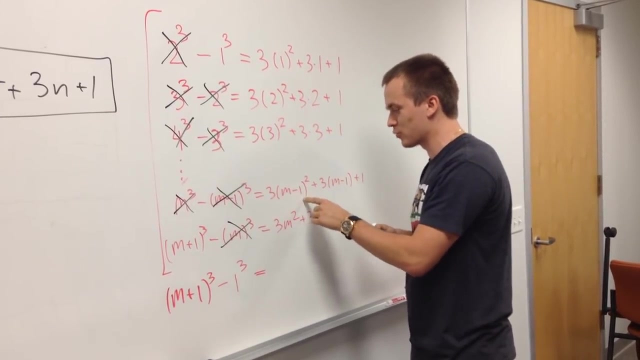 What I will get. I will get m plus one cube minus one cube equal. What about right hand side? In right hand side, you can see, three is a common number for all these terms And I have one square, two square, three square, m minus one square, etc. 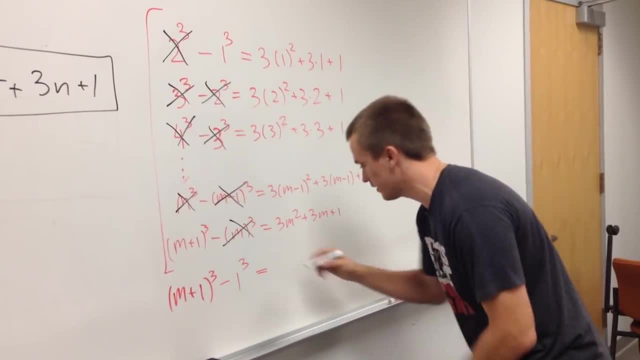 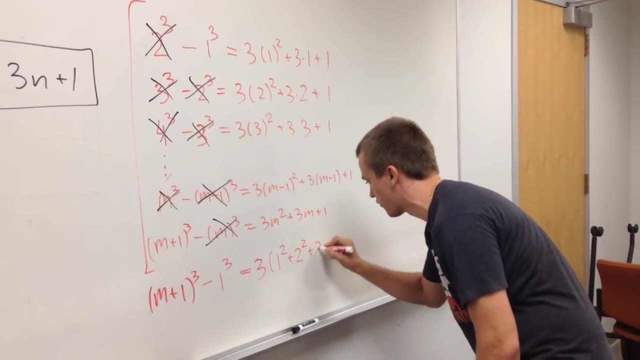 And this is my goal, And I'm going to factor three. So on the right hand side I will have three. I'm going to factor three, One square plus two square plus three square plus m square, And this is sum that we want to find. 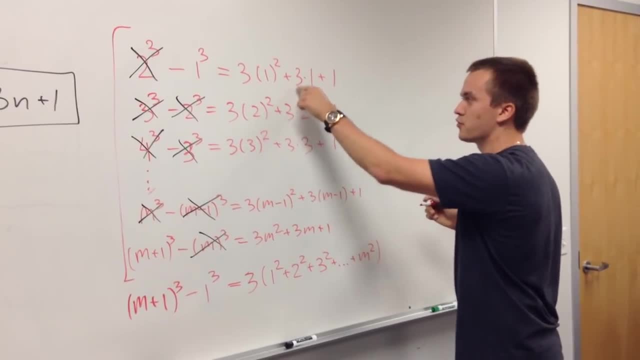 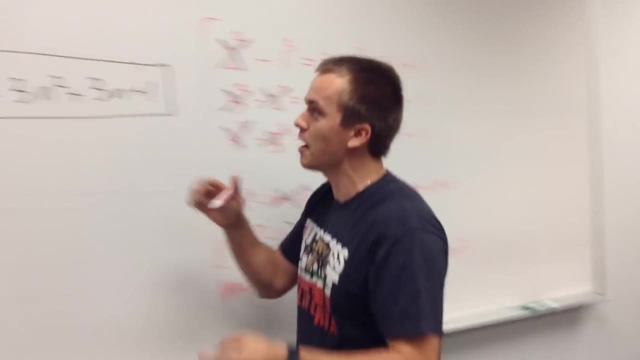 But what else we are left with? We're left with three. We're going to factor three. It's going to be one plus two plus three plus m minus one plus m. But this sum, we know This is going to be m and m times m plus one over two. 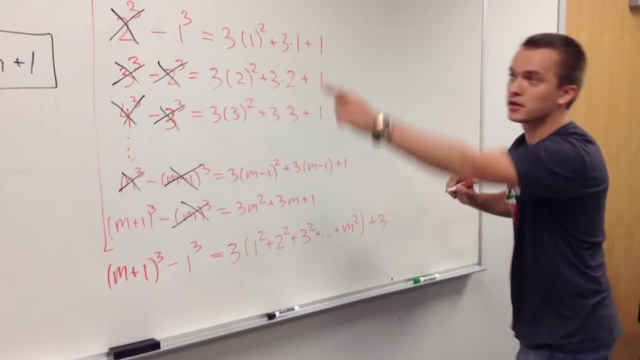 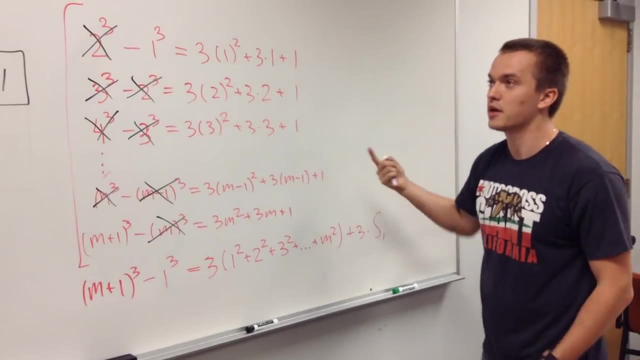 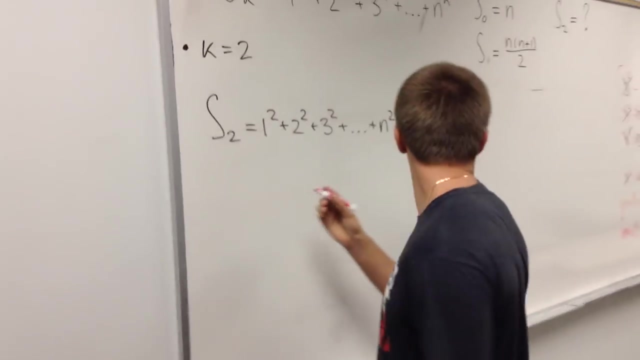 So here we will have three, And this sum is equal to s one. And what is this? one plus one plus one n times n times is just going to be s zero. So m plus s zero. Okay, So what we know? 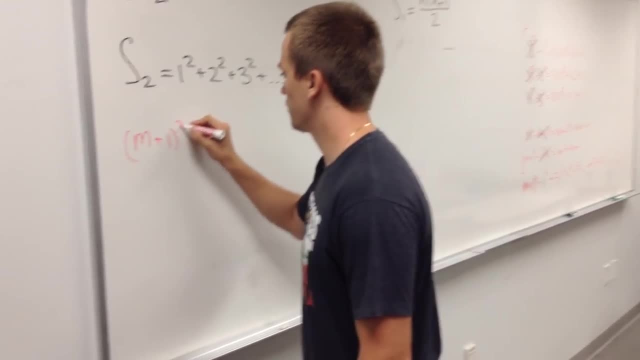 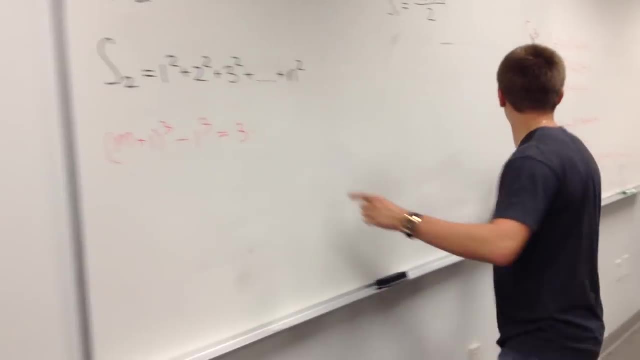 What we got? We got that m plus one cube minus one cube, equal to three, And let's name this one as s two, And this is my goal that I want to find This is s two And this is my s one. 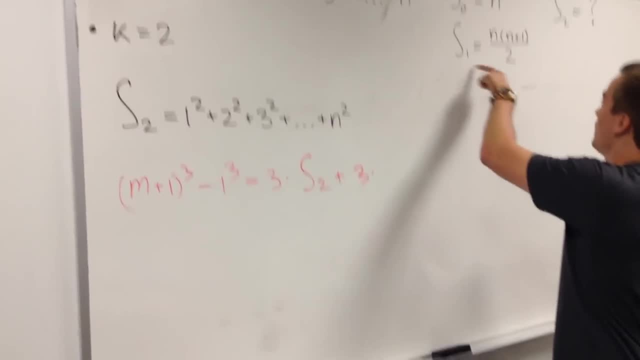 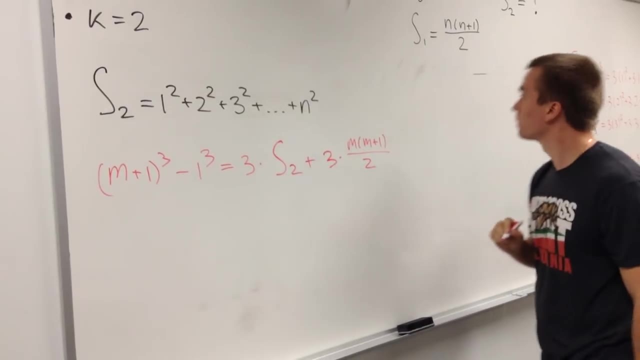 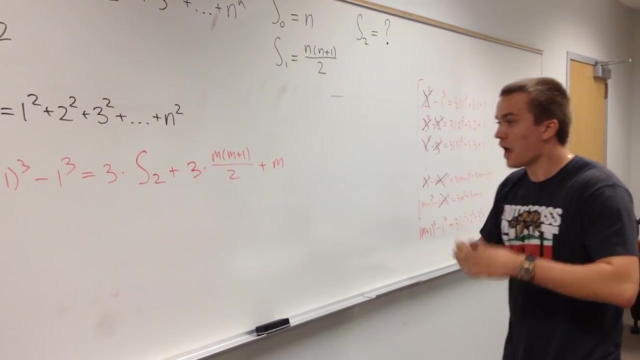 My s one is three times s one. In our case is n equal to m. So I have m m plus one over two And plus s zero And s zero is n. So plus m, And right now you can see an amazing thing. 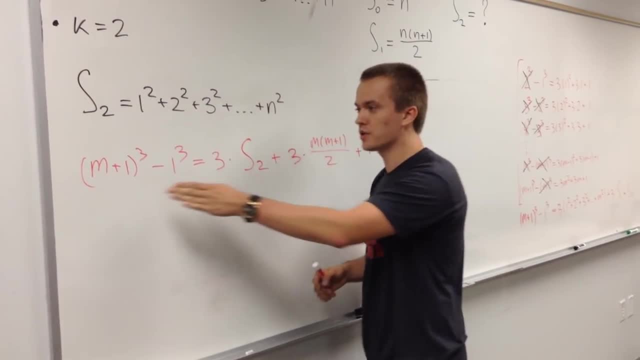 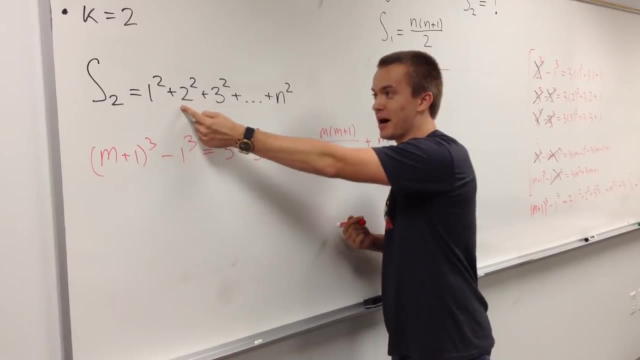 We Our known is s two, We know this is our m, We have numbers. So right now we can solve this equation for s two And we will get the sum. We will get expression in terms of m for this sum. So let's do it. 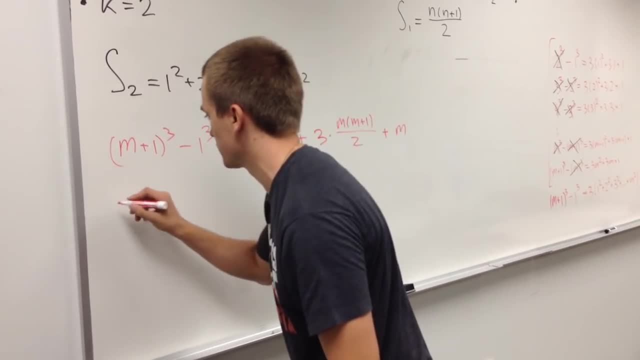 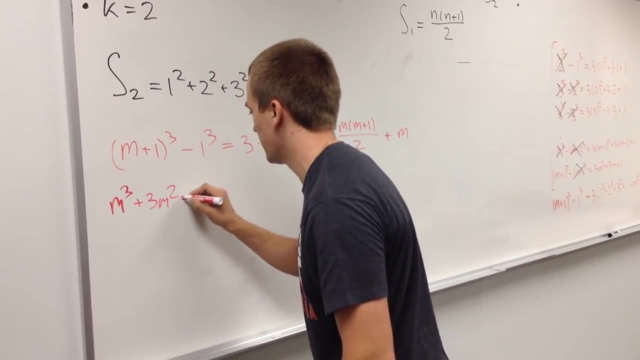 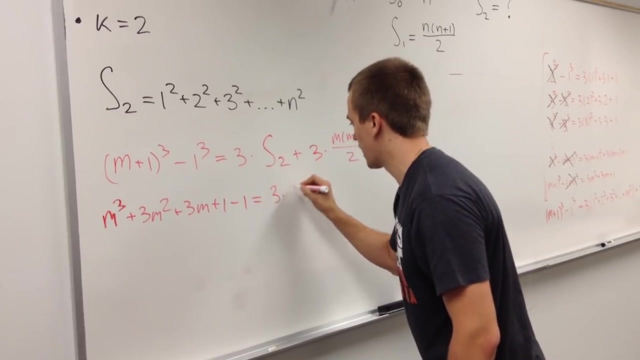 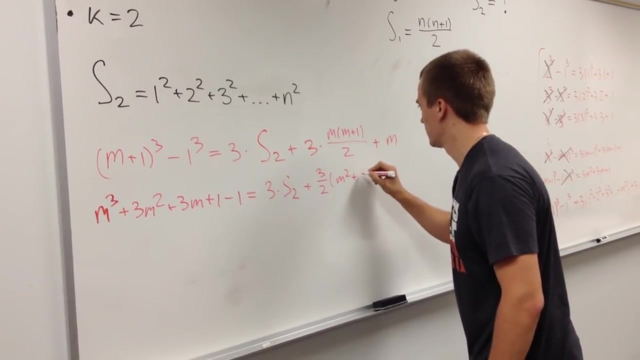 Let's first find m plus one cube minus one. So it's going to be m cube plus three m square plus three m plus one minus one. Yeah, What I will get here. Here I will get three times s two And plus three half m square plus m. 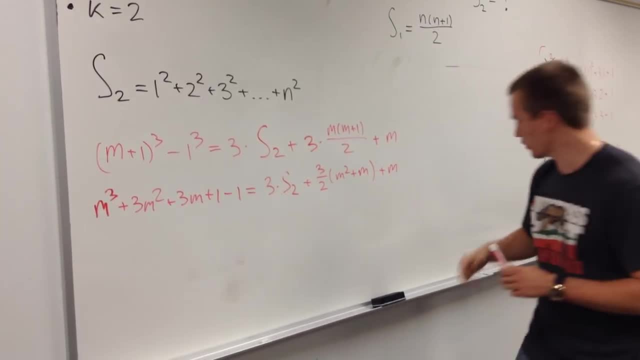 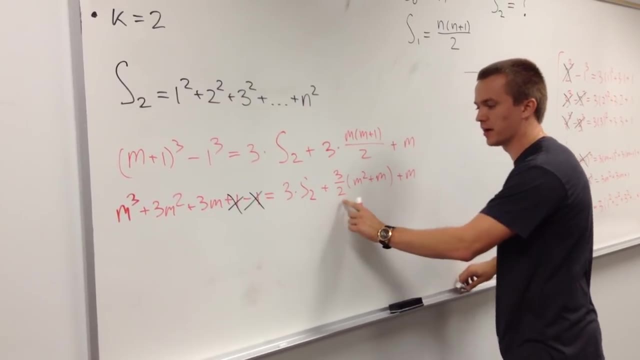 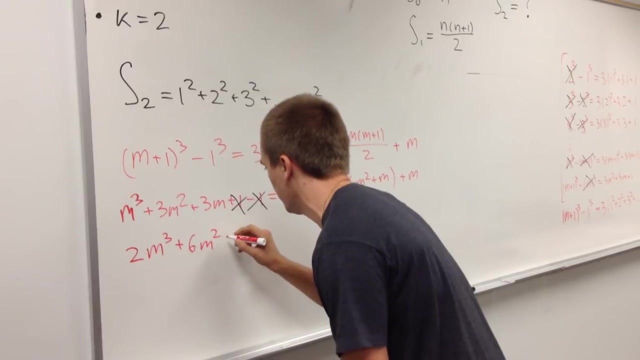 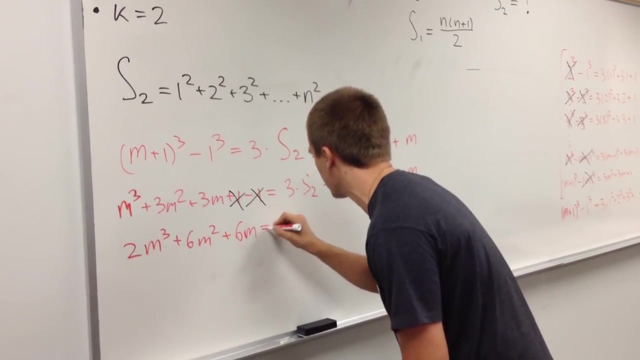 Plus m. Yeah, So here one got cancelled, And let's multiply both sides by two, So what I will get? I will get two m cube plus six m square plus three, Oh, not three Plus six m Plus six m. 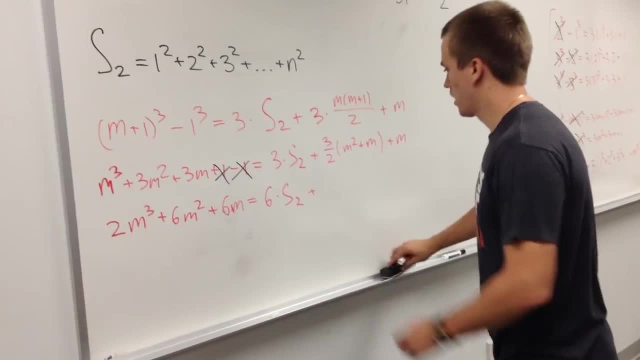 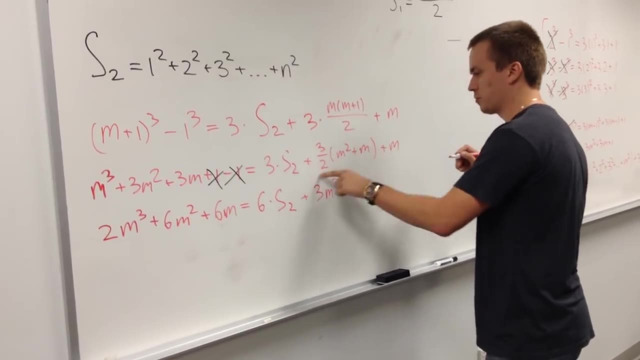 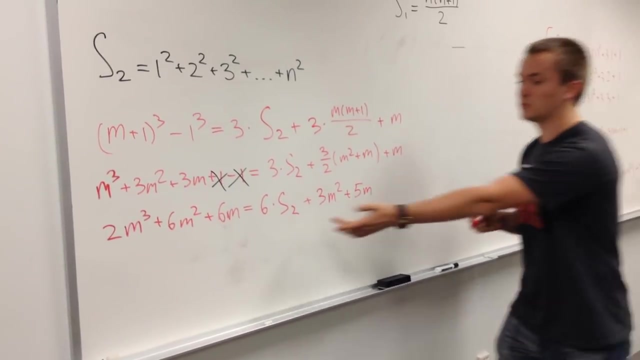 Equal six times s two, And also multiply by two, We have three m square, Three m plus, Remember, we multiply by two. So it's two m, Two m plus three m, It's going to be plus five m. So, and let's right now solve this for s two.